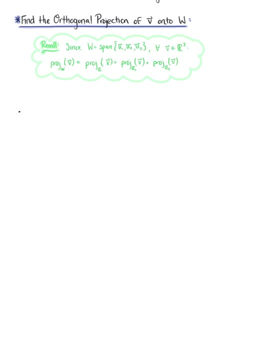 and then taking their sum. So here's our scratch work. We have the projection of vector V onto vector U sub one, which we know, by definition, is the dot product of vector U sub one with vector V, divided by the dot product of vector U sub one with itself. 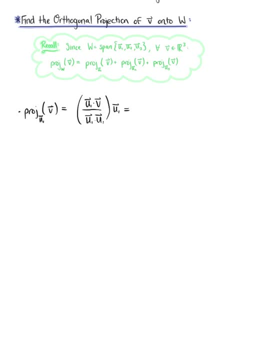 multiplied by vector U sub one, So we have the dot product of vector U sub one, which is defined as one, one, zero, zero. And we're dotting this with the given vector V, which has the components four negative three. 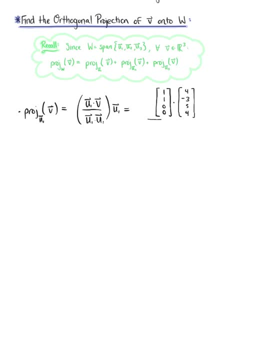 five, four, And then this is all divided by the dot product of vector U sub one with itself. So this is our scalar multiple multiplied by vector U sub one. So, computing these dot products in the numerator, we have four minus three plus zero plus zero. 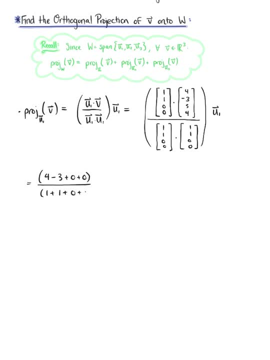 all divided by one plus one plus zero plus zero, All divided by one plus one plus zero plus zero, Multiplied by vector U sub one. So our scalar multiple is one half. And now we're ready to multiply this by the vector U sub one. 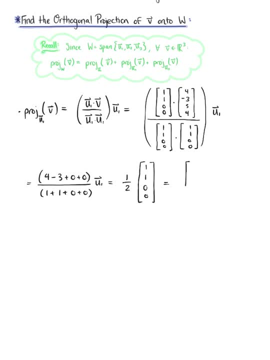 one one, zero, zero. So our first projection is the vector with components one half, one half, zero, zero. So now we're moving on to the second projection, And this is the projection of vector V onto vector U, sub two. 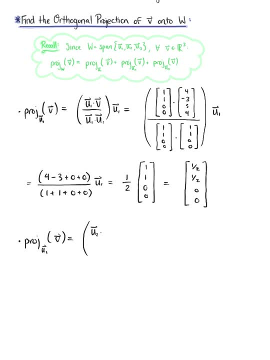 So by definition we know that this is the dot product of vector U sub two, with vector V, all divided by the dot product of vector U sub two, with itself Multiplied by vector U sub two. So our scalar multiple, we have the dot product of vector U sub two. 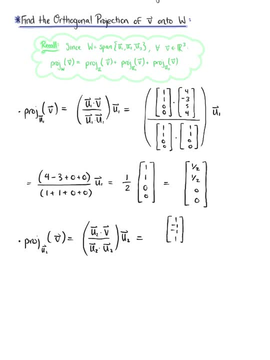 which is one negative one, negative one, one, And we are dotting this with vector V, So that's four negative three, five, four, And this is all divided by the dot product of vector U, sub two with itself. 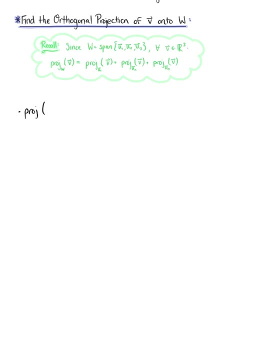 So here's our scratch work. We have the projection of vector v onto vector u sub 1, which we know, by definition, is the dot product of vector u sub 1, with vector v divided by the dot product of vector u sub 1, with itself multiplied by vector u sub 1.. 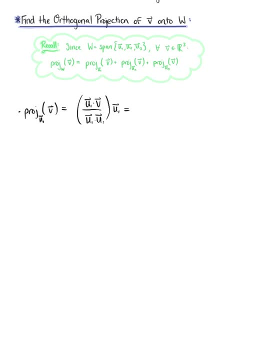 So we have the dot product of vector u, sub 1, which is defined as 1, 1, 0, 0, and we're dotting this one It's with the given vector v, which has the components 4, negative, 3,, 5,, 4,, and then this: 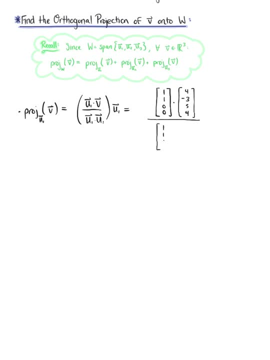 is all divided by the dot product of vector u sub 1 with itself. So this is our scalar multiple multiplied by vector u sub 1.. So, computing these dot products in the numerator, we have 4, minus 3, plus 0, plus 0. 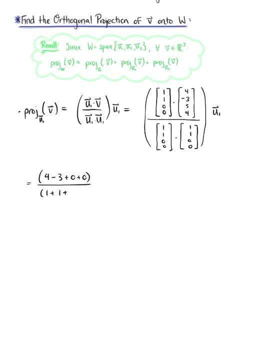 All divided by 1, plus 1, plus 0, plus 0,, multiplied by vector u sub 1.. So our scalar multiple is 1 half, and now we're ready to multiply this by the vector u sub 1, 1, 1, 0, 0. 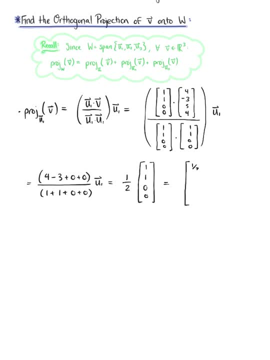 So our first projection is the vector with components 1, half, 1 half, 0, 0.. So now we're moving on to the second projection: 1, 1, 0, 0.. And this is the projection of vector v onto vector u, sub 2.. 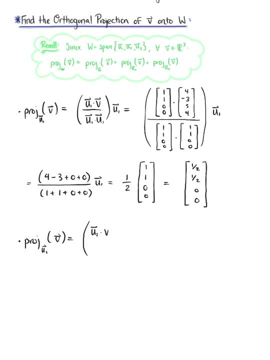 So by definition, we know that this is the dot product of vector u sub 2, with vector v, all divided by the dot product of vector u sub 2, with itself multiplied by vector u sub 2.. So our scalar multiple, we have the dot product of vector u sub 2, which is 1, negative 1,. 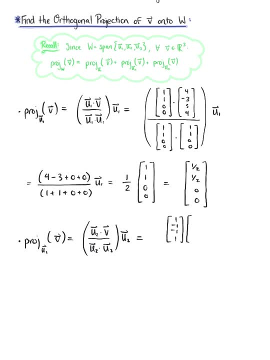 negative 1, 1.. And we are dotting this with vector v, So that's 4, negative 3, 5, 4.. And this is all divided by the dot product of vector u, sub 2, with itself. 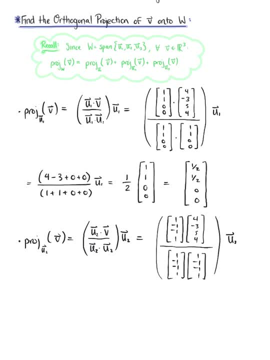 Again, this is all multiplied by vector u sub 2.. So, computing these dot products in the numerator, we have 4, plus 3, minus 1, minus 0, 1, 1, minus 5, plus 4.. 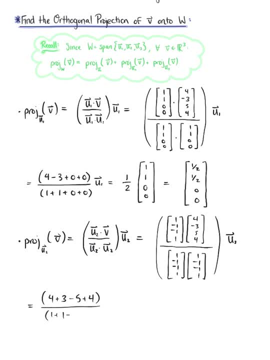 And in the denominator we are left with 1 plus 1 plus 1 plus 1, multiplied by vector u sub 2.. So this is going to simplify to the scalar: multiple 3 halves multiplied by vector u sub 2.. 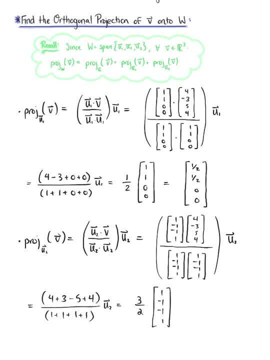 So 1 negative 1, negative 1, 1.. And distributing that scalar multiple through, we have the vector with components: 3 halves negative, 3 halves negative, 3 halves positive, 3 halves Beautiful And last but not least, 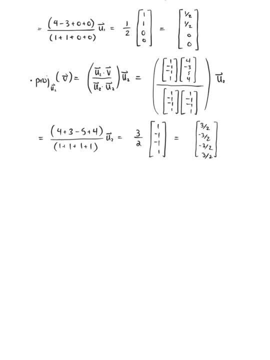 we need to consider the projection of vector v onto u sub 3.. So by definition, we know that this is the dot product of vector u sub 3, with vector v divided by the dot product of vector u sub 3, with itself all multiplied by vector u, sub 3.. 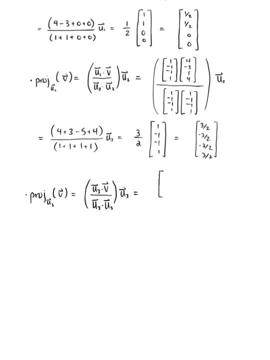 So vector u, sub 3, is the vector with components 0,, 0,, 1,, 1.. And we dot this with vector v, which has components 4, negative, 3,, 5,, 4.. And this is all divided by the dot product of the vector 0,, 0,, 1,, 1 with itself. 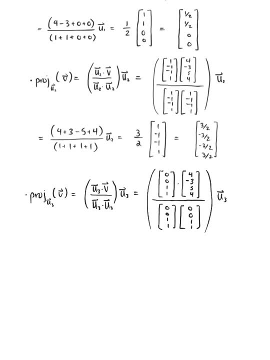 And remember that's just the scalar multiple. so we're multiplying this by vector u, sub 3.. And computing these dot products, in the numerator we have 0 plus 0 plus 5 plus 4.. And in the denominator we have 0 plus 0 plus 1 plus 1, multiplied by vector u, sub 3.. 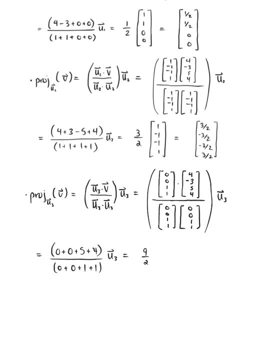 So our scalar multiple is 9 halves multiplied by vector u sub 3, which is the vector u sub 3.. Which is the vector with components 0,, 0,, 1,, 1.. And distributing that scalar, we are left with the vector with components 0, 0,, 9 halves, 9 halves. 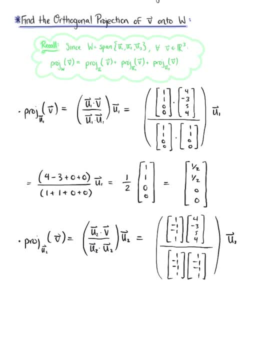 Again, this is all multiplied by vector U sub two. So, computing these dot products, in the numerator we have four plus three minus five plus four, And in the denominator we are left with one plus one plus one plus three, 1 plus 1, multiplied by vector u sub 2.. So this is going to simplify to the scalar multiple. 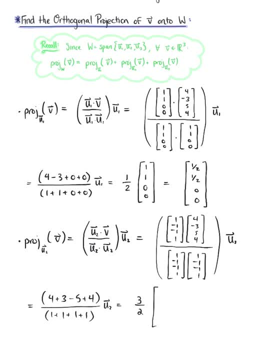 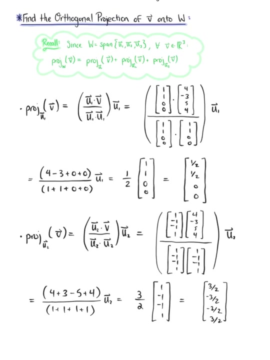 3 halves multiplied by vector u sub 2.. So 1, negative, 1, negative, 1, 1.. And distributing that scalar multiple through, we have the vector with components: 3 halves negative, 3 halves negative, 3 halves positive, 3 halves Beautiful. And last but not least, we need 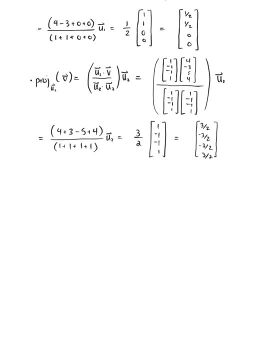 to consider the projection of vector v onto u sub 3.. So by definition we know that this is the dot product of vector u sub 3 with vector v divided by the dot product vector v of vector u sub 3, with itself all multiplied by vector u sub 3.. 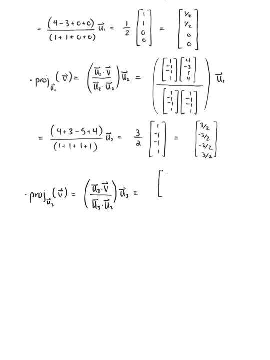 So vector u, sub 3, is the vector with components 0,, 0,, 1,, 1.. And we dot this with vector v, which has components 4, negative, 3,, 5,, 4.. And this is all divided by the dot product of the vector 0,, 0,, 1,, 1 with itself. 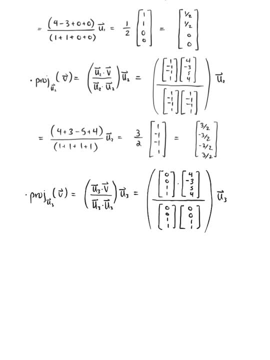 Now remember that's just the scalar multiple. so we're multiplying this by vector u, sub 3.. And computing these dot products, in the numerator we have 0 plus 0 plus 5 plus 4.. And in the denominator we have 0 plus 0 plus 1 plus 1, multiplied by vector u, sub 3.. 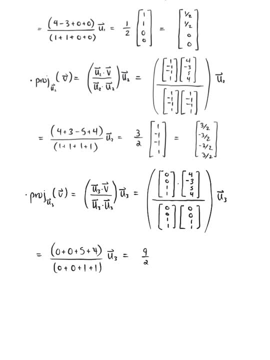 So our scalar multiple is 9 halves multiplied by vector u sub 3, which is the vector with components 0,, 0,, 1,, 1.. And distributing that scalar, we are left with the vector with components 0,, 0,, 9 halves. 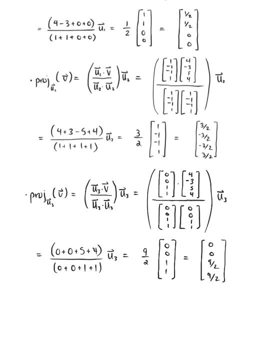 9 halves Phew. So we are officially ready to find the full projection. So we can say that therefore, the projection of vector v onto subspace w is equal to. so our first vector, the first projection. So the projection equation of vector v onto u, sub 1, was 1, 1,, 0,, 0, and we're adding: 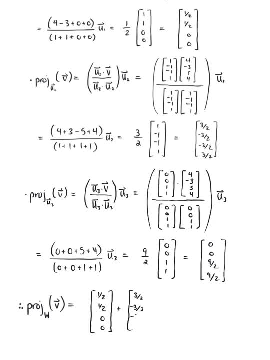 this to the projection of vector v onto u, sub 2, which has components 3, 2, 5 minus 3, 2, 5 minus 1, 0, 13, minus 1, 0, 0, 72.. 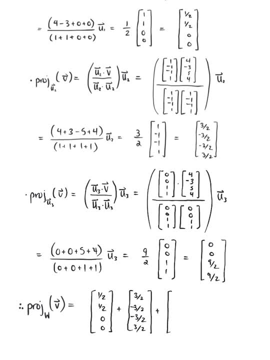 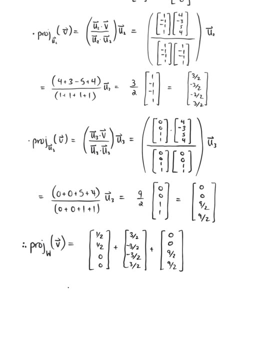 And we add this to the projection of vector v onto u, sub 2, which has components 0, 2, 0.. which is 3, 2, 0,. just that, 9 halves. and combining up those like terms, we are left with a beautiful final answer. 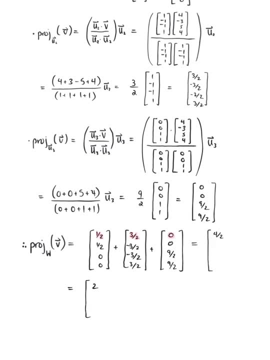 We have 1 half plus 3 halves is 4 halves or 2.. We have 1 half minus 3 halves, which is minus 2 by 2, or negative 1.. We have negative 3 halves plus 9 halves, which leaves us with 6 halves or 3.. 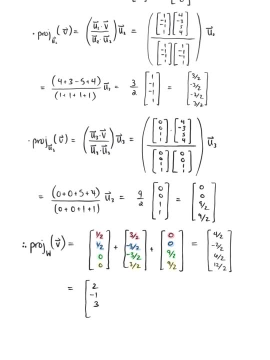 And last but not least, we have 3 halves plus 9 halves, which is 12 halves or 6.. And so there you have it. This is our beautiful final answer. 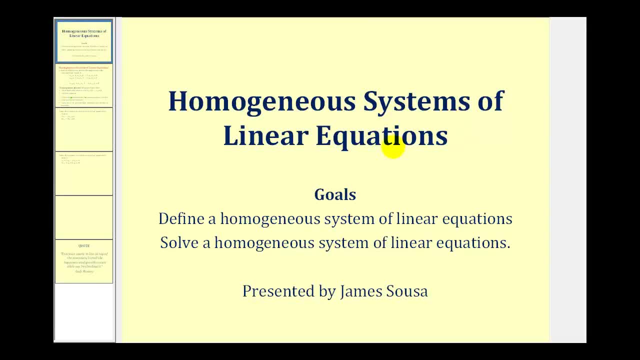 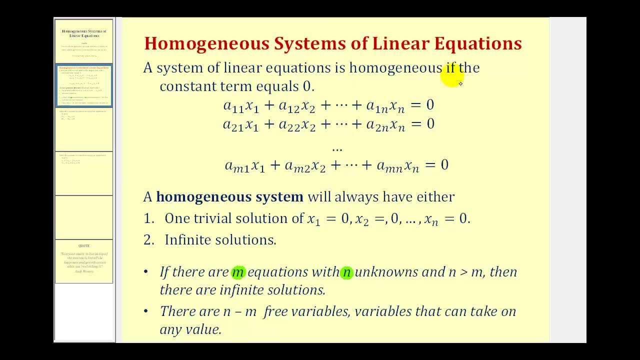 Welcome to a lesson on homogeneous systems of linear equations. The goals of the video are to define a homogeneous system of linear equations and also to solve a homogeneous system of linear equations. A system of linear equations is homogeneous if the constant term equals zero, Meaning the system must fit this form here. 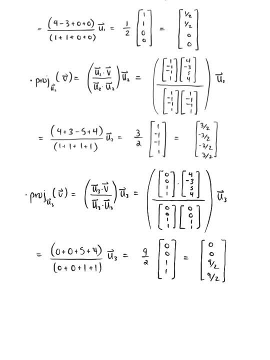 Phew, So we are officially ready to find the full projection. So we can say that therefore, the projection of vector v onto subspace w is equal to. So our first vector, the first projection, vector v onto u, sub 1, was 1 half, 1 half, 0, 0. 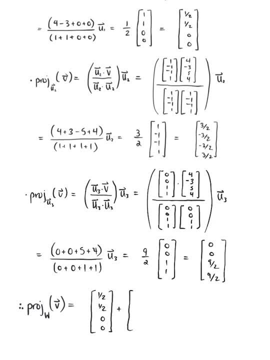 And we are adding this to the projection of vector v onto u, sub 2, which has components: 3 halves minus 3 halves minus 3 halves positive 3 halves plus the projection of vector v onto u sub 3,. 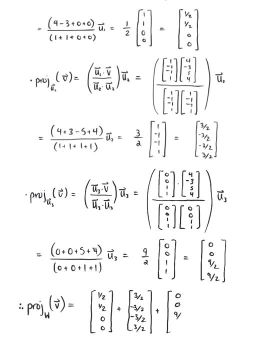 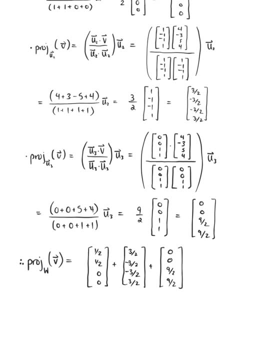 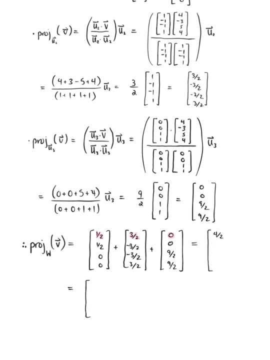 which is the vector, with components 0,, 0,, 9 halves, 9 halves, And combining up those like terms, we are left with a beautiful final answer. We have 1 half plus 3 halves: is 4 halves or 2.. 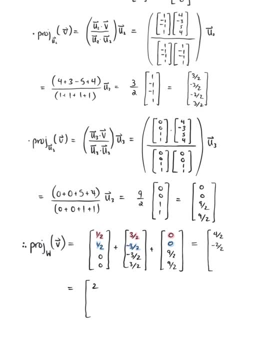 We have 1 half minus 3 halves, which is minus 2 by 2, or negative 1.. We have negative 3 halves plus 9 halves, which leaves us with 6 halves or 3.. And, last but not least, we have 3 halves plus 9 halves, which is 12 halves or 6..